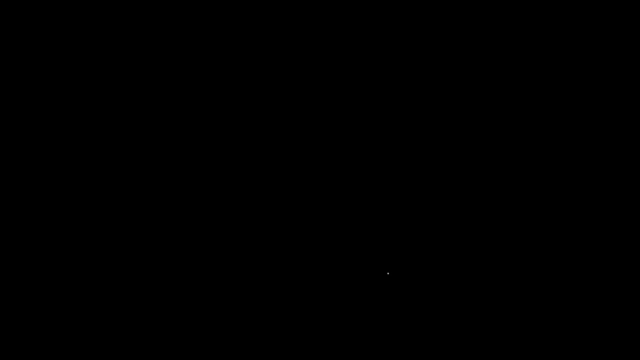 In this video, we're going to focus on graphing rational functions using transformations. So let's start with this function: 1 over x. The curve exists in quadrants 1 and 3.. So this is quadrant 1, and here we have quadrant 2,, this is quadrant 3, and this is quadrant 4.. 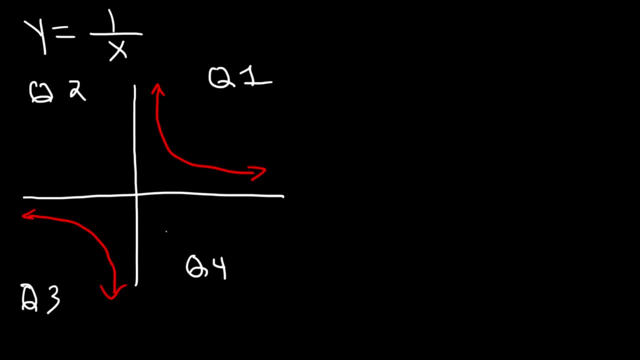 Now, what are the vertical and horizontal asymptotes of this graph? The vertical asymptote is basically the y-axis. The vertical asymptote is: x is equal to 0.. You can find it by setting the denominator equal to 0.. So that's the vertical asymptote. 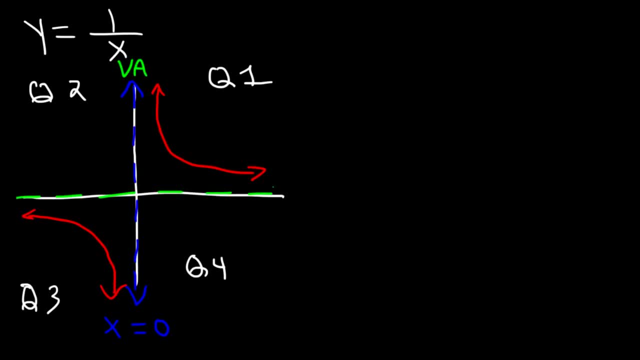 The horizontal asymptote is the x-axis and the equation is: y is equal to 0.. Now, what about the graph negative 1 over x? How is it different from the graph on the left? The only difference is it reflects over the origin, so to speak. 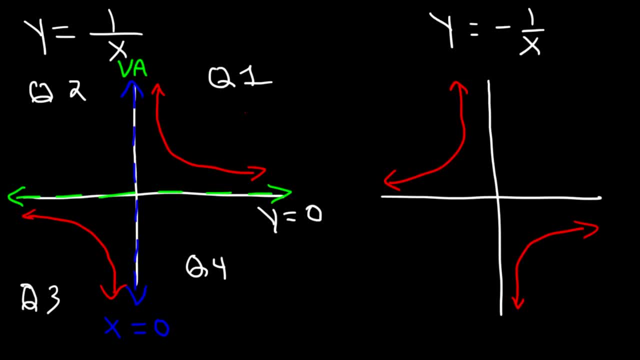 Well, technically you can see it as a reflection over the y-axis. This side switches to this side, which we can see it here, And this side switches over here. You can also describe it as a reflection over the x-axis, because if you take this side and move it here, it looks like this portion. 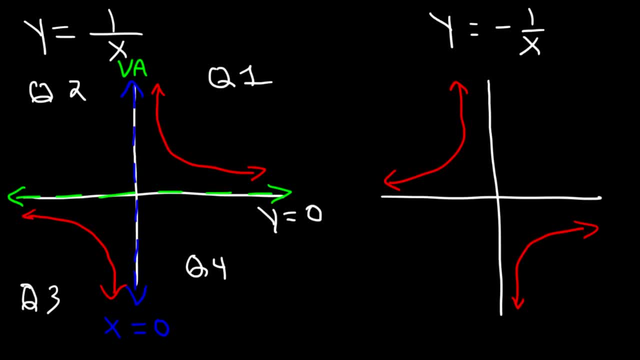 The vertical asymptote and the horizontal asymptote are the same for these two graphs, So what's the domain and the range? for the graph on the left, The domain includes all possible x values. The only thing that you need to remove from the domain in this example is the horizontal asymptote. 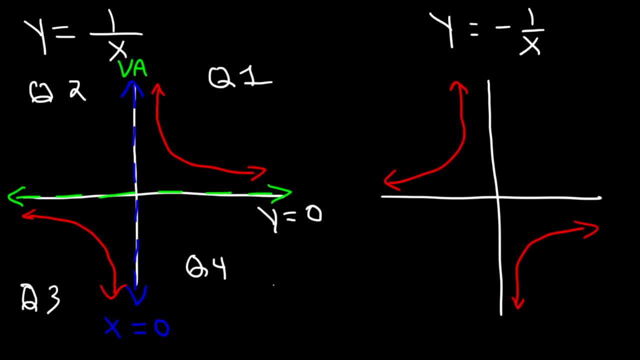 The only thing that you need to remove from the domain in this example is the vertical asymptote, which is: x equals 0.. If you plug in 0, the function is undefined. That's why the curve does not exist there. So the domain includes every x value except 0. 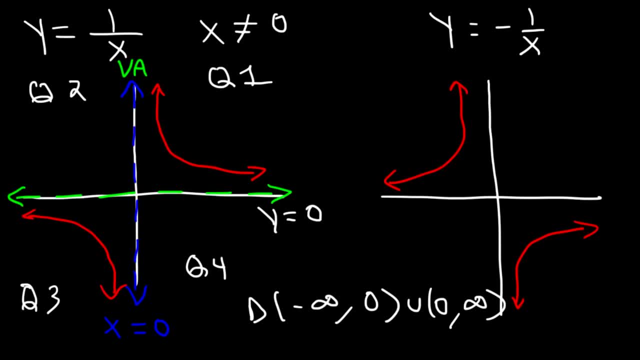 So it's from negative infinity to 0, union 0 to infinity. Now for the range. you need to remove the horizontal asymptote, So the range is going to be the same as as the domain. So, as we've seen in the last example, 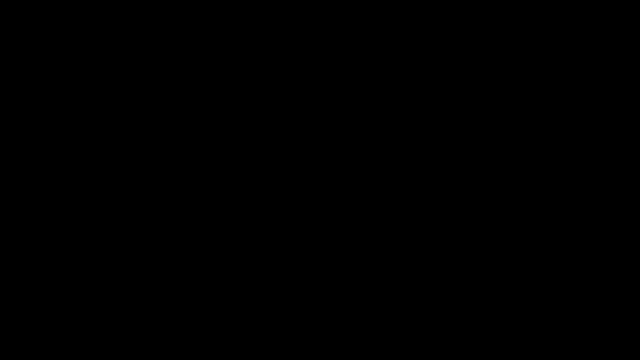 1 over x and negative 1 over x were symmetric about the origin, which means they're odd functions. Now, what about this graph? 1 over x squared And also negative 1 over x squared. What do you think? the general shape? 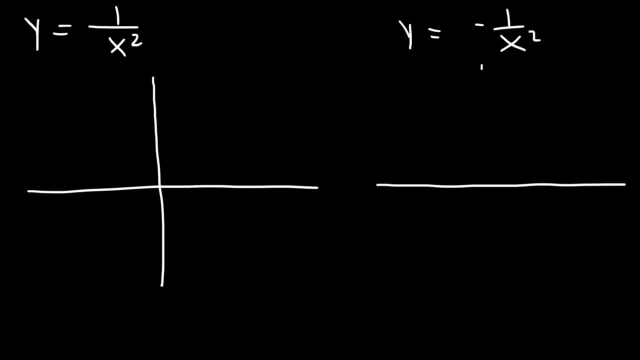 for these two graphs will look like. So these two graphs still have a vertical asymptote at x equals 0, and also a horizontal asymptote at y equals 0.. But they're going to be even functions. They're symmetric about the y-axis. 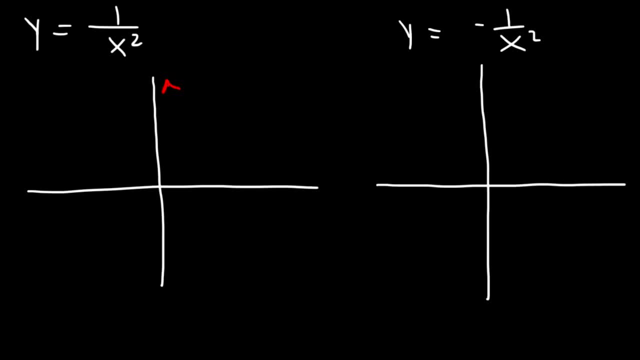 which is the vertical asymptote. So the first one is going to exist above the x-axis, Because 1 over x squared is always positive. If you were to replace x with negative 5 and then square it, that would be positive 25.. 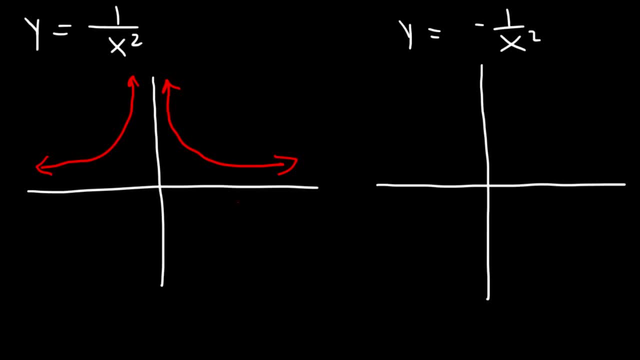 So it's always going to be positive or above the x-axis. Negative 1 over x squared is going to reflect over the x-axis But, as you can see, it's still symmetric about the y-axis, which means that these two functions. 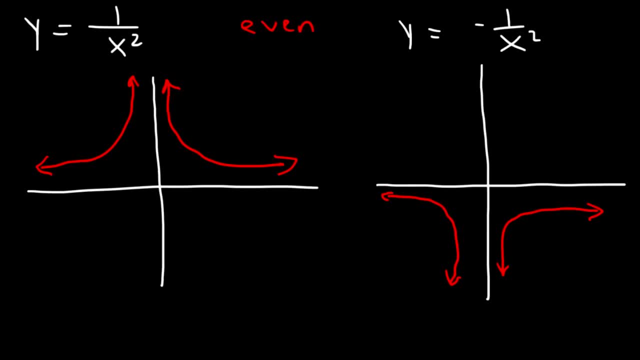 are even functions. The domain for both graphs will be the same. It's negative infinity to 0, union 0 to infinity. So the way you find a domain is you start from the left side- negative infinity- and the graph continues all the way to the right side. 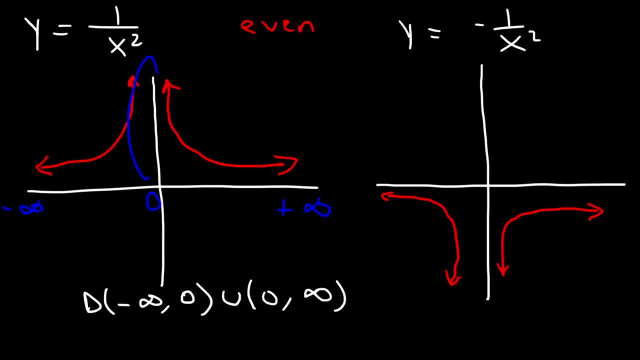 However, it doesn't touch 0.. As you can see, there's the red line never intersects the x-value of 0. It never touches the y-axis, So you have to remove 0 from the domain. Now, the range of these two functions are not the same. 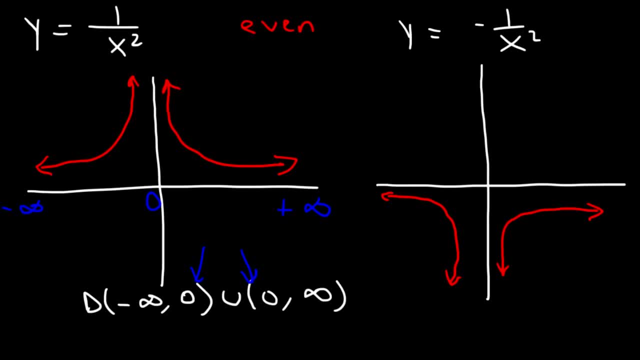 What is the range for the first one. So, when dealing with the range, you have to look at the y-values. The lowest y-value is 0,. the highest is infinity. So the range is going to be 0 to infinity And it does not include 0,. 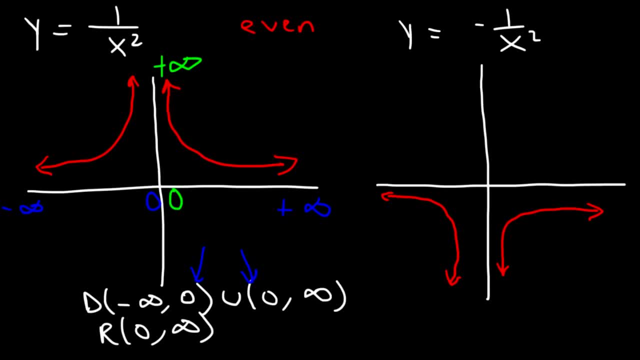 so you need to use parentheses instead of brackets. Now, what about the range? for the graph on the right, Notice that the lowest y-value is negative infinity and the highest is 0.. So it's going to be negative infinity to 0.. 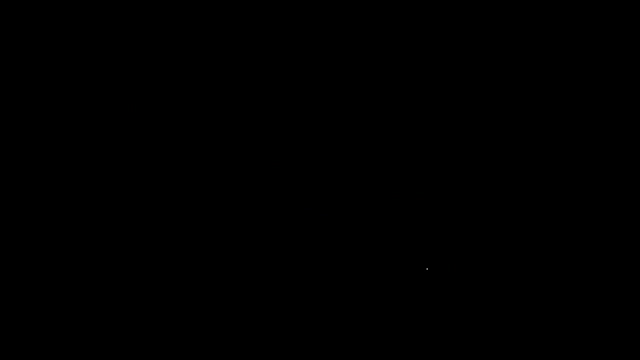 That's the range, And 0 is not included. Now what about this graph? 1 over x plus 2.. How can we graph it? This graph is going to look similar to 1 over x, but it's going to shift 2 units to the left. 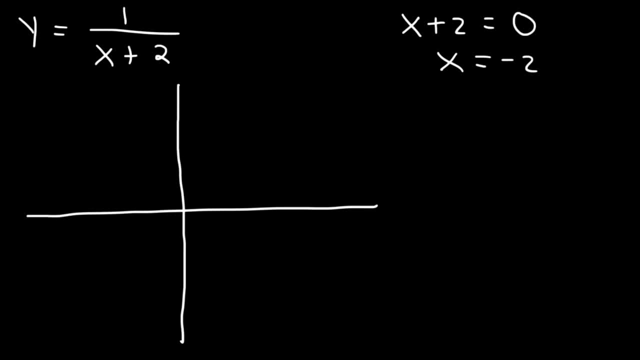 If you set the denominator equal to 0,, you'll see that x is equal to negative 2.. That is the vertical asymptote. So let's plot that first. And we know that 1 over x exists in quadrants 1 and 4.. 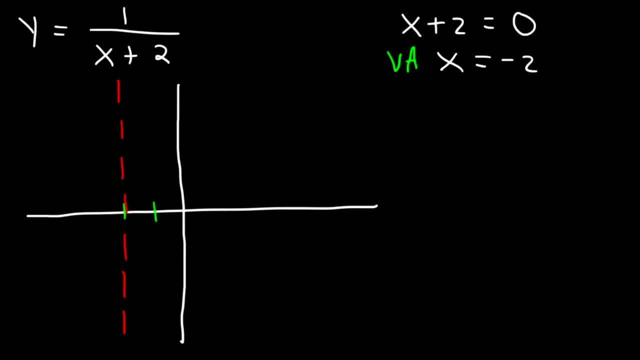 So, relative to the vertical asymptote, it's going to exist in the upper right section and the lower left section. So that's going to be the graph of 1 over x plus 2, using transformations. Now, if you want to get an accurate sketch, 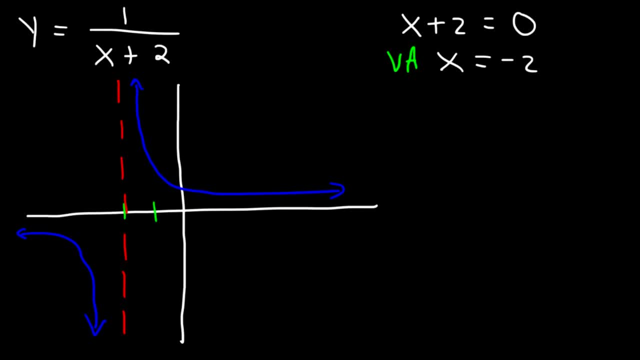 you can plug in points, but my focus is not that in this lesson. I just want to focus on the general shape. So, now that we have the general shape, what's the domain and what's the range? So the lowest x value is negative infinity. 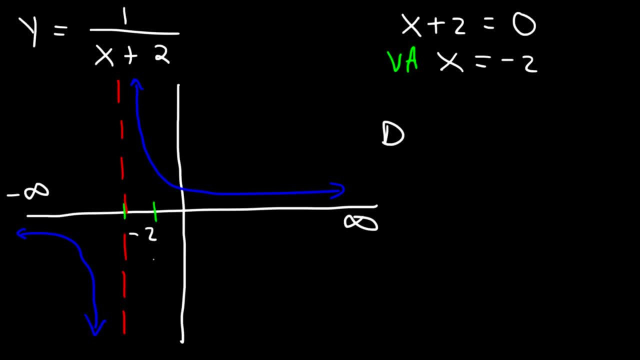 The highest is infinity. And we have to take out the vertical asymptote negative 2.. Because if the vertical asymptote is negative 2, that means in the function x cannot equal negative 2.. It will be undefined because you'll get a 0 in the denominator. 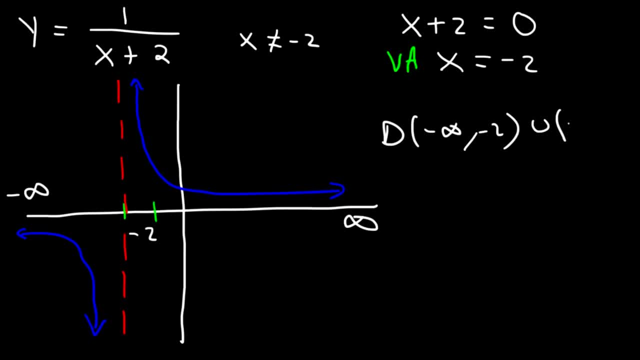 So the domain is going to be from negative infinity to negative 2 union, negative 2 to infinity, And the horizontal asymptote is still: y equals 0. It hasn't changed, Which means that y varies from negative infinity to positive infinity, But it doesn't include the horizontal asymptote. 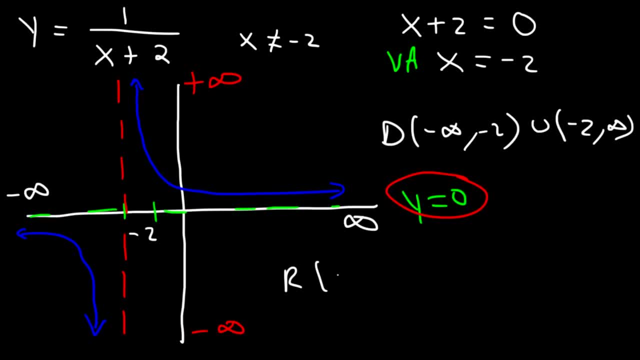 The curve doesn't touch it, So the range is negative: infinity to 0. union 0 to infinity. So keep this in mind: Always remove the horizontal asymptote from the range And remove the vertical asymptote from the domain. Let's try this one. 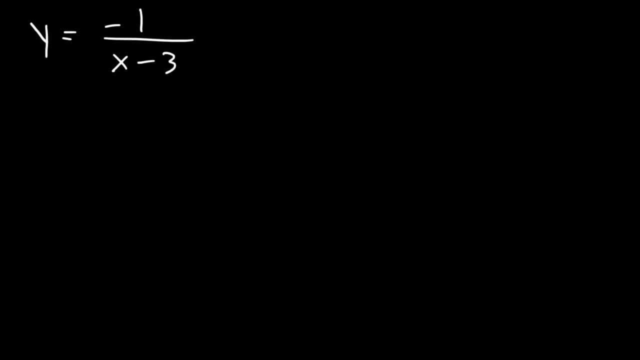 Negative: 1 over 2 over x minus 3.. So what kind of transformations do you see in this graph? There's two of interest. x minus 3 means that the graph, the vertical asymptote, is going to shift 3 units to the right. 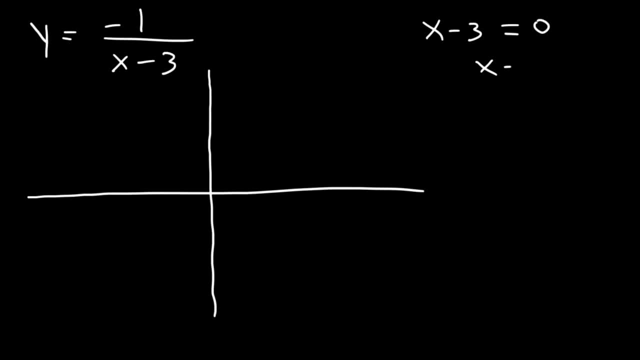 If you set the denominator equal to 0,, you'll see that the vertical asymptote is: x is equal to 3.. That's the first transformation, Which is basically a horizontal shift Right 3 units. Now we have a negative in front of the function. 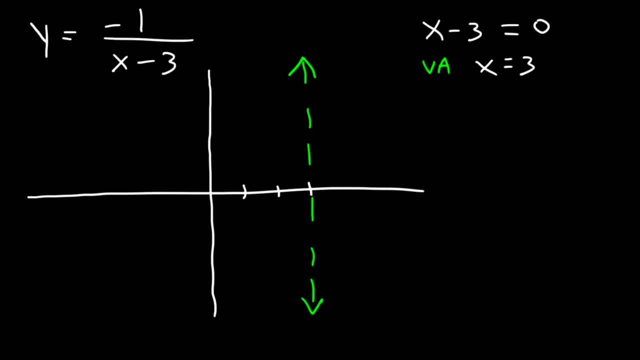 So that means that it's going to- you could say, reflect over the x axis, if you want to. So 1 over x will typically exist in the upper right and upper left section, But it's going to flip This part instead of being at the top. 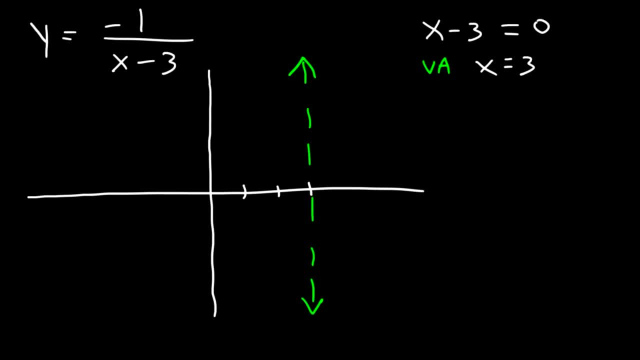 is now going to be at the bottom, So it's going to exist here and here, And that's just a rough sketch. It's not an accurate sketch. I didn't plot any points, Just a simple rough sketch. So now, what are the domain and range? 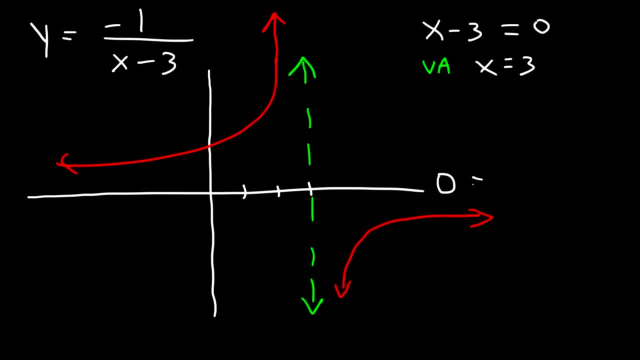 of this function, We know the range is going to be the same. The horizontal asymptote is: y is equal to 0. And y can vary from negative infinity to infinity, But it doesn't include 0. The range hasn't changed in this example. 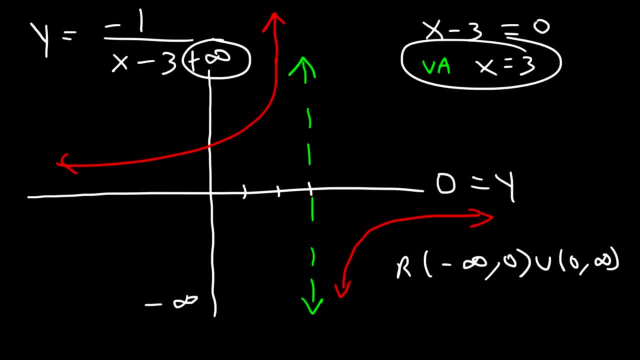 But the domain has, because the vertical asymptote has changed. The lowest x value is negative infinity, The highest is positive infinity And we need to take out 3, which is the vertical asymptote. So the domain is going to be from negative infinity to 3.. 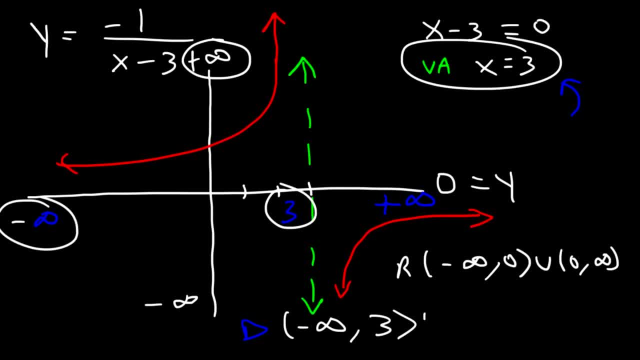 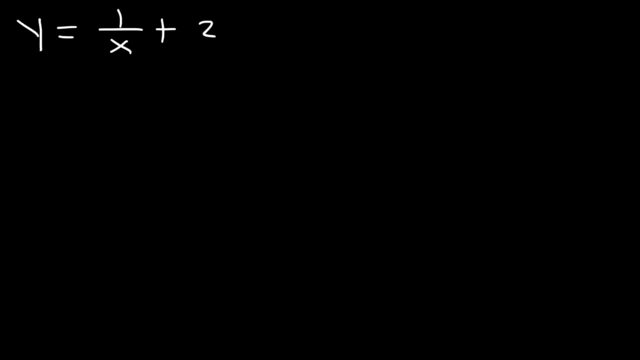 You view it from left to right and then union this side. The right side is from 3 to infinity, Not including 3.. Consider this one: 1 over x plus 2.. How can we graph it? What type of transformations exist? 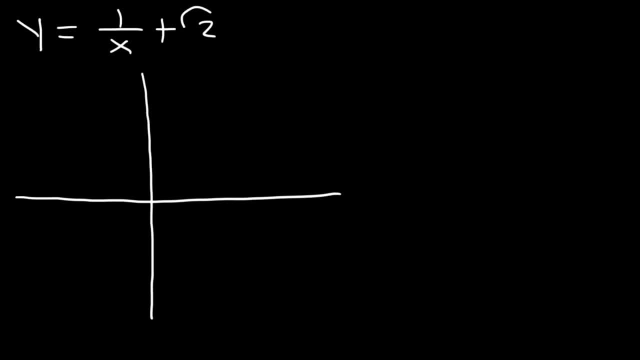 in this graph. So the plus 2 means that it's going to shift up 2 units. Now we know that for 1 over x, the horizontal asymptote is y is equal to 0.. So if we add 2 to it, it's going to be. 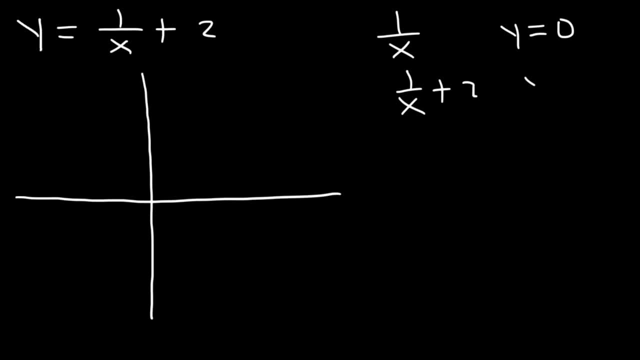 0 plus 2.. So therefore, the horizontal asymptote is: y is equal to 2.. It's basically this number here that you see. So whatever that constant is out in front, that's going to be the horizontal asymptote. The vertical asymptote is based on this number. 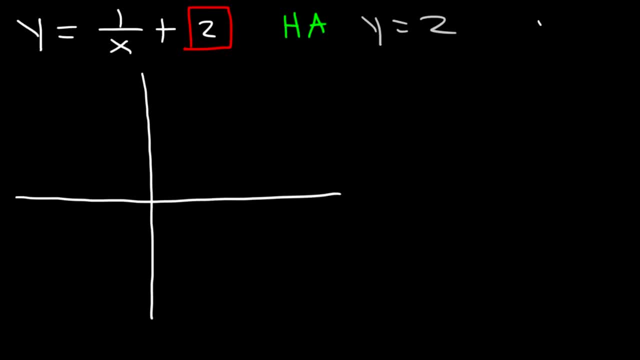 or that variable. If x is equal to 0, well, x will be equal to 0.. So that's the VA or the vertical asymptote. So let's plot the asymptotes. So the horizontal asymptote is that y is equal to 2.. 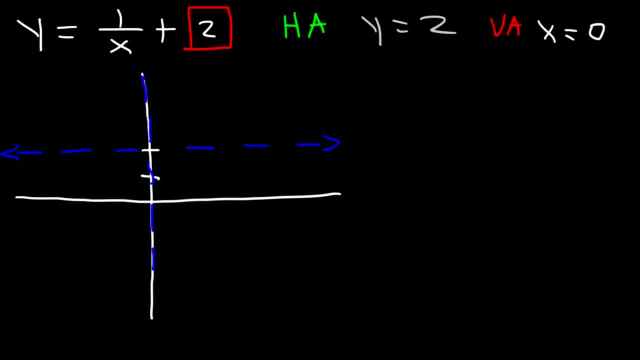 And the vertical asymptote is the y-axis, which x is equal to 0.. Now it's positive 1 over x. So, like 1 over x, it's going to exist in the upper right corner and the lower left corner. Now what's? 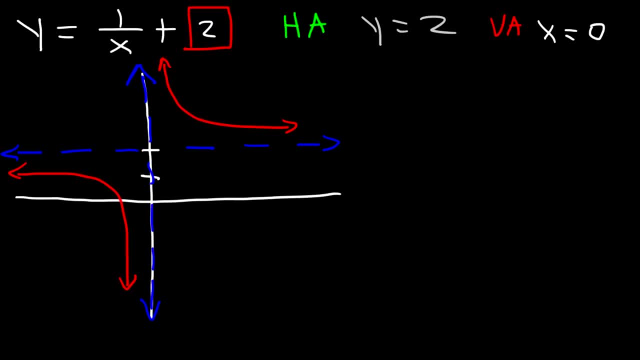 the domain and what's the range for this function. So, starting with the domain, the lowest x value is negative infinity. It's going to stop at the vertical asymptote, which is x is equal to 0.. And the highest x value is infinity. 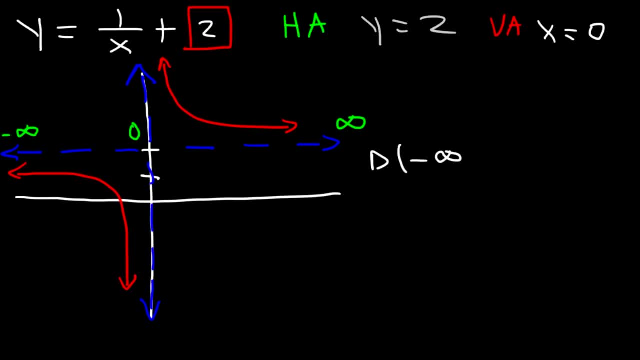 So the domain is going to be from negative infinity to 0, union 0 to infinity. Now, what about the range? The lowest y value that we see is negative infinity, And then it's going to stop at 2,, which is the horizontal asymptote. 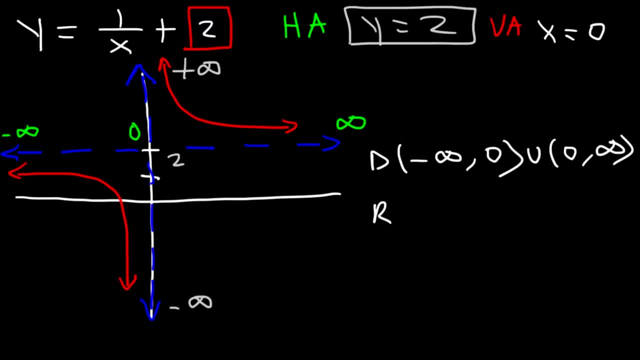 And the highest y value is positive infinity. So the range is going to be from negative infinity to 2, union 2 to infinity. So always remember to remove the horizontal asymptote from the range. Now let's move on to our next example. 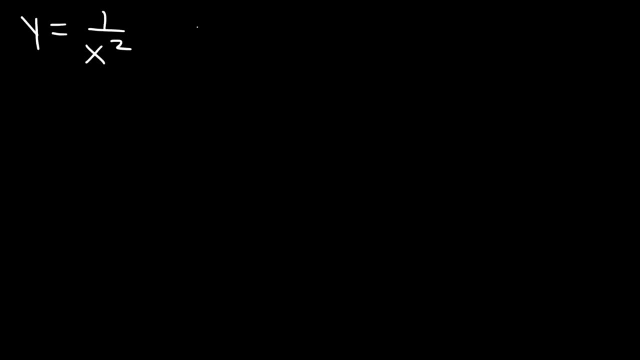 Let's try: 1 over x, squared minus 3.. So how can we graph this function? So we can see that the horizontal asymptote is based on the constant negative 3.. So it's y is equal to negative 3.. And if we set the denominator? 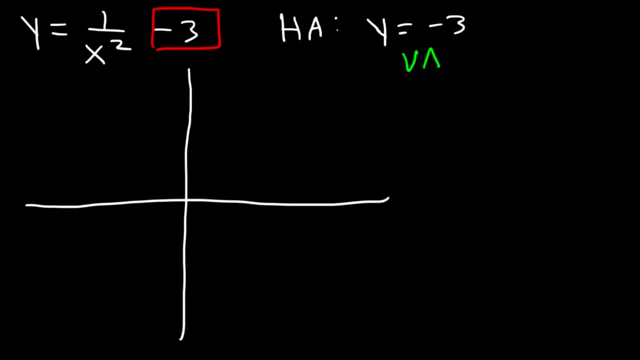 equal to 0, we'll get the vertical asymptote, which is simply: x is equal to 0.. So that's everything that we have so far. So let's plot the vertical asymptote, which is just the y-axis, And let's plot the 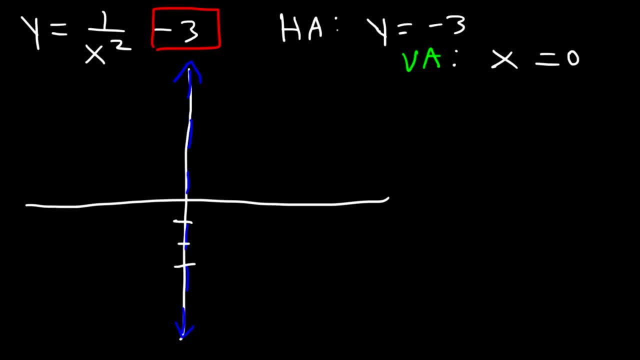 horizontal asymptote which is at y, equals negative 3.. So here's the horizontal asymptote And this is positive: 1 over x squared. 1 over x squared is going to be symmetric about the vertical asymptote which is, in this case, 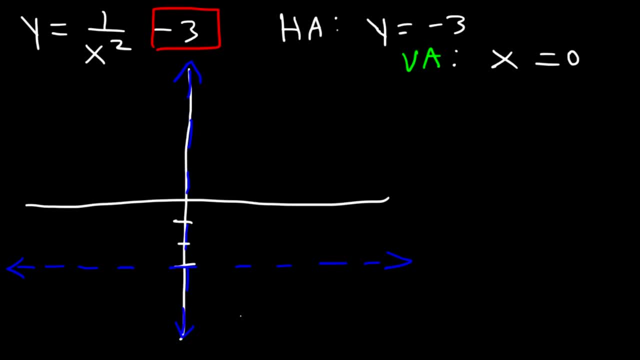 the y-axis. It's an even function and because it's positive, it's going to be above the horizontal asymptote. So it's going to look like this: It's the same as 1 over x squared, but it's been shifted down. 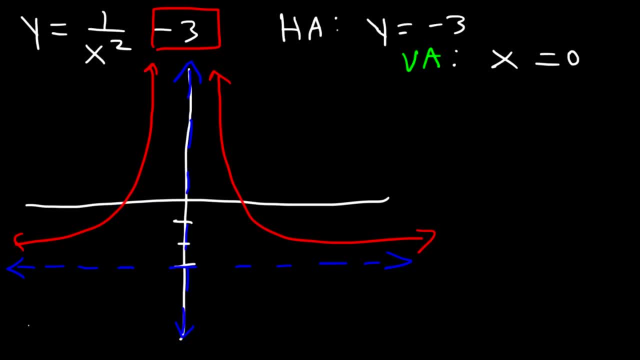 3 units. So what's the domain and range of the function? So, analyzing the domain, the graph starts from the left- negative infinity- it stops at the vertical asymptote and it continues all the way to the right, to positive infinity. 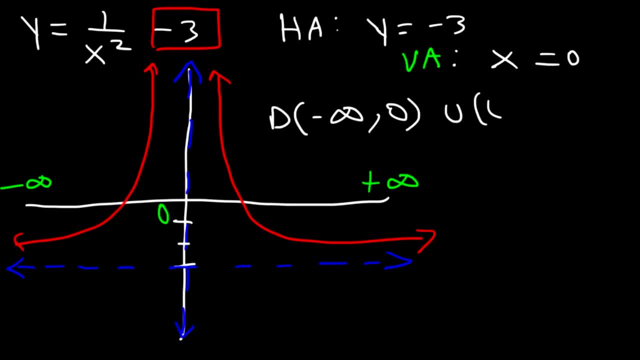 So it's negative infinity to 0, union 0 to infinity. As for the range, notice that the lowest y-value is negative 3, and the highest is positive infinity. So the range is from negative 3 to infinity, And that's it for this. 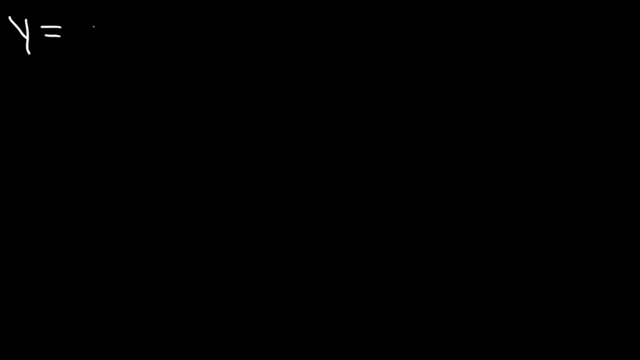 example, Try this problem: 3 minus 1 over x plus 2.. So, using everything you know, go ahead and draw a rough sketch, Identify the horizontal and the vertical asymptote and also write the domain and range using interval notation. 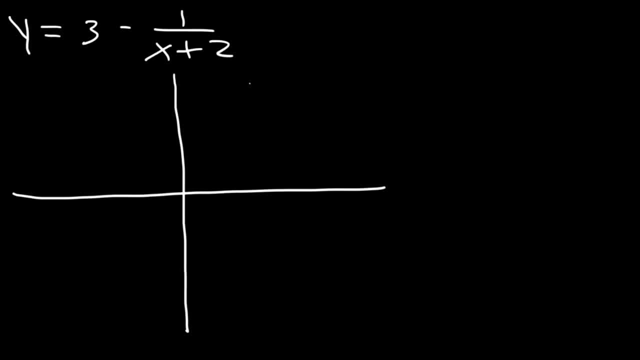 So let's start with the horizontal asymptote. So we can see that we have a constant 3 in front. so it's going to be: y is equal to positive 3.. And for the vertical asymptote, if we set x plus 2, equal to 0,. 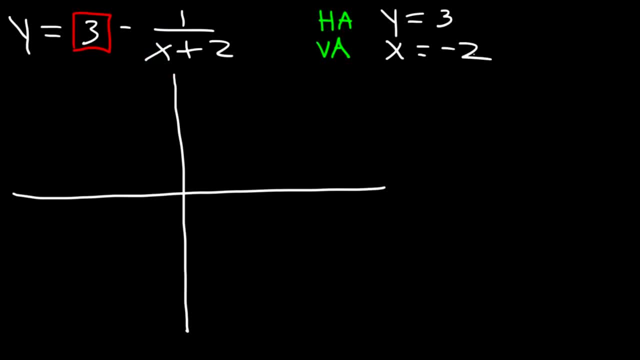 x will be equal to negative 2.. So therefore, the graph shifts 2 units to the left and up 3 units. So this is: the vertical asymptote at x equals negative 2.. And then we have the horizontal asymptote at y. 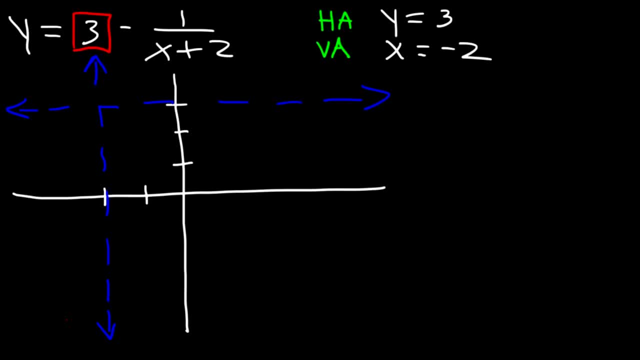 equals 3.. So here's a question for you: Will the graphs, will this graph exist in the upper right corner and the lower left corner, Or will it exist in the upper left corner And the lower right corner? what would you say? 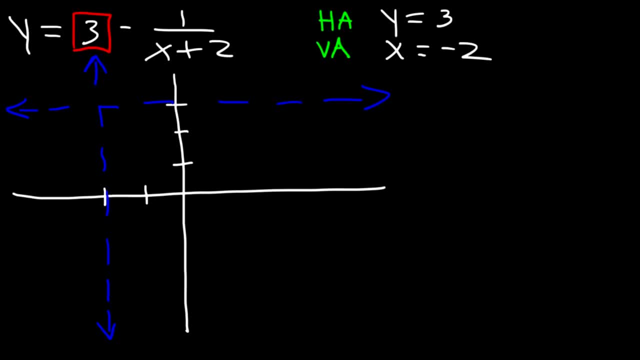 So is it similar to 1 over x or negative? 1 over x. Notice the negative in front. So it's going to reflect over the horizontal asymptote. so relative to 1 over x. So it's going to exist in the upper left corner. 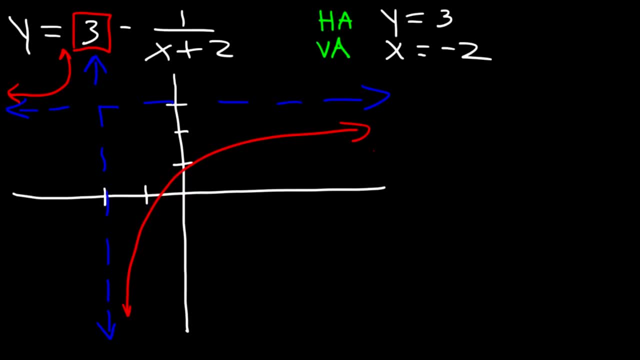 and the lower right corner. Now, with this information, what is the domain and the range of the function? So, starting with the domain, the lowest x value is negative infinity, the vertical asymptote is negative 2, and the highest is infinity. 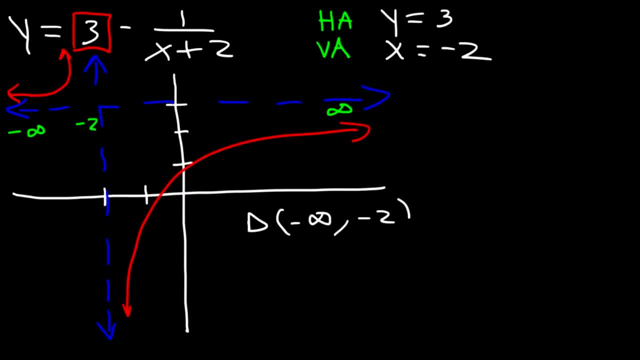 So the domain is going to be from negative infinity to negative 2, union, negative 2 to infinity. As for the range, you can see that the lowest y value is negative infinity, the horizontal asymptote is positive 3, and the highest y value is 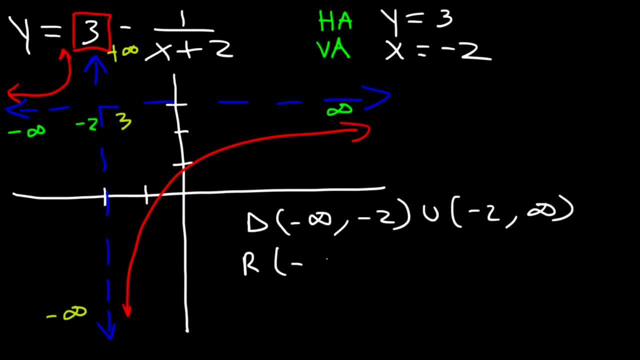 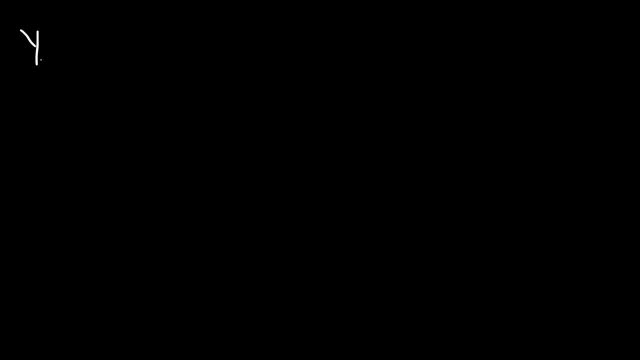 positive infinity. So the range is going to be negative: infinity to 3, union 3 to infinity. Let's try this one: y is equal to 3 divided by 1 over x minus 2 squared. So what is the horizontal asymptote? 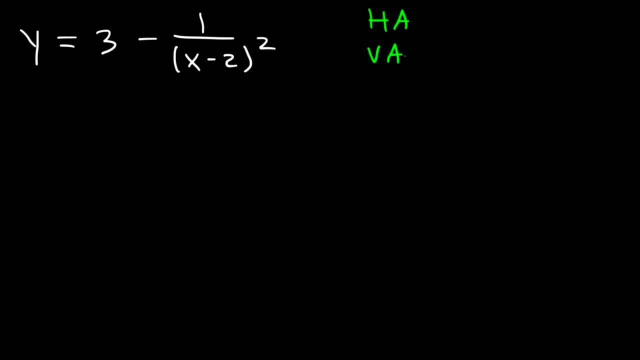 and what is the vertical asymptote? So the horizontal asymptote is based on that number, So it's going to be positive 3 again. And the vertical asymptote, if we set x minus 2 equal to 0, then we can see that x.